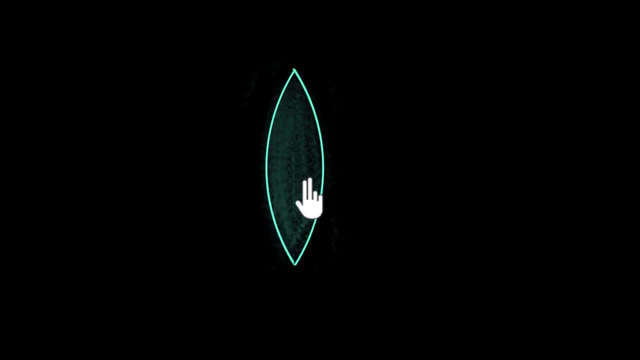 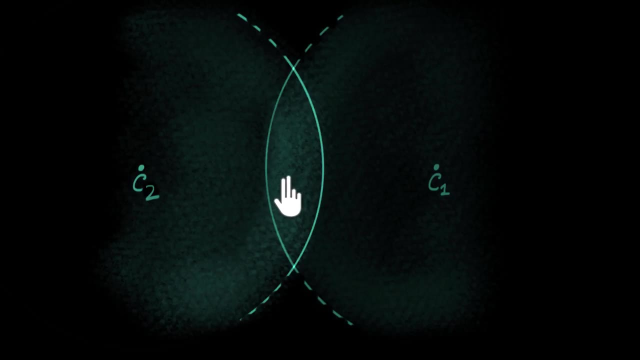 In our example, we have both the surfaces to be curved, And these surfaces are spherical surfaces, which means they're both parts of a sphere. And a lens is called as a thin lens if the thickness of that lens is much smaller, much smaller than the radius of curvature. 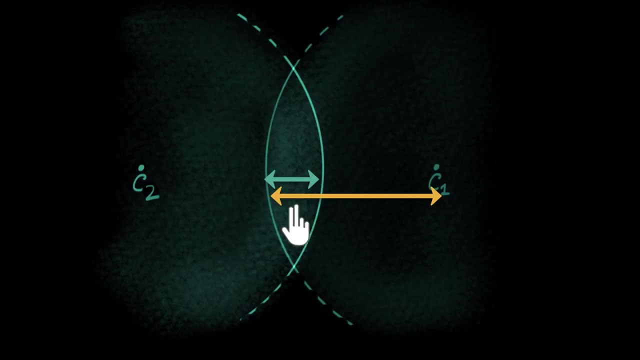 of each of that sphere. Now, of course, in this diagram the thickness doesn't look all that small. I've exaggerated the thickness And we've done that because it'll be easier to draw the ray diagrams and show the ray diagrams. But we'll assume, but we'll just assume, that this thickness is actually. 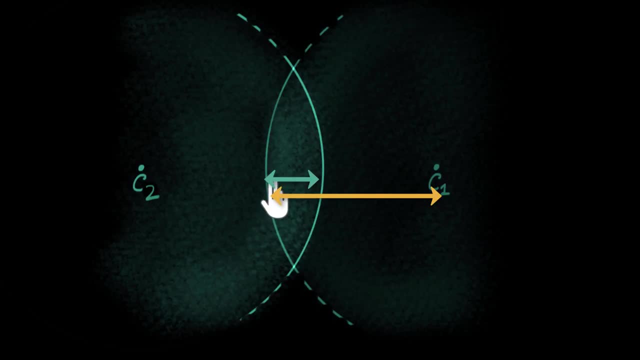 way smaller than the radius of curvature, Then we'll call that as a thin lens, And our goal now is to figure out what is the focal length of such a thin lens. So let's draw our principal axis, And O is just the center of this thin lens. We usually call it as the. 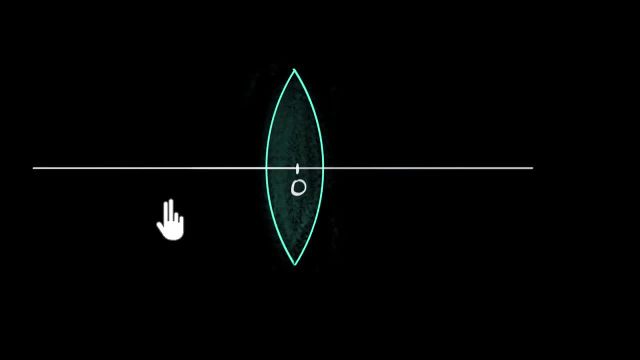 optic center And, just like for curved mirrors, to figure out the focal length, we're going to draw parallel rays of light and see where they meet up. One ray of light will draw along the principal axis. Since this ray of light is perpendicular to both the surfaces, the 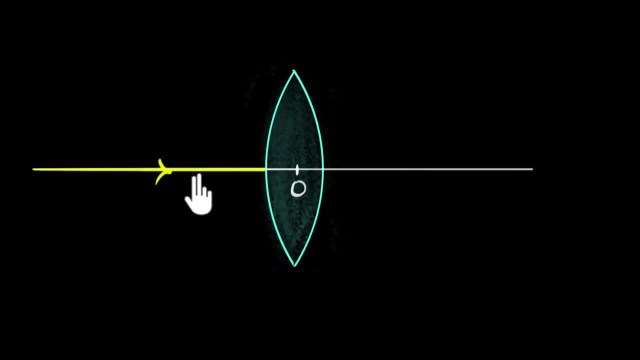 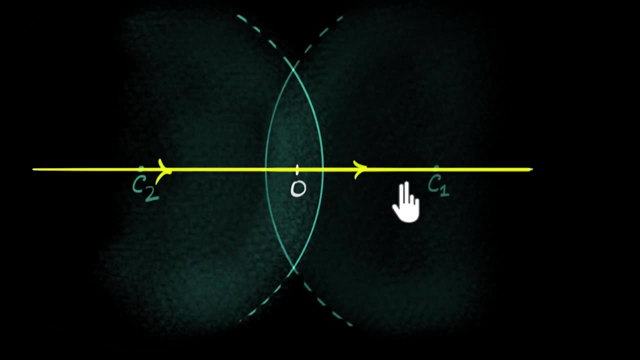 angle of incidence is zero, There'll be no refraction, And so this ray will go undeviated. How do we know it's perpendicular to the surface? Well, notice that the ray of light is passing through the centers of curvature, and any line through the center of curvature is always 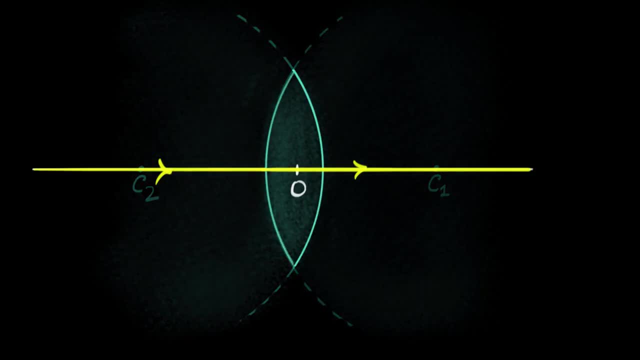 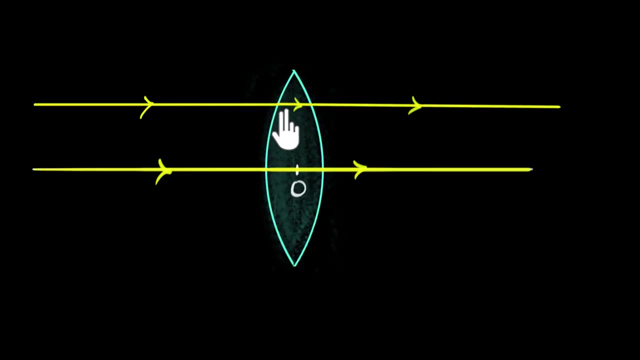 perpendicular to the surface. So this ray goes undeviated. The second ray of light will draw above the principal axis. Now this ray of light will refract, it will bend. and to figure out how it bends, let's first focus on the first curved surface. So we'll 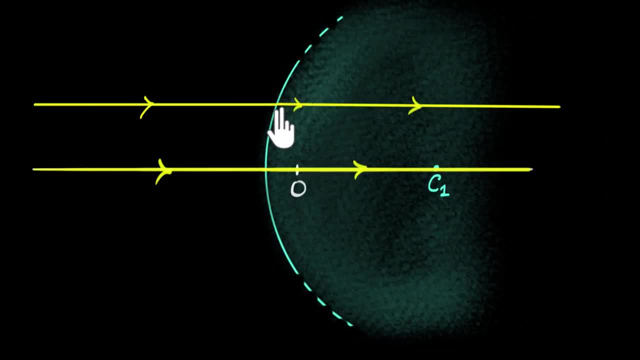 assume the second surface is not there for a while. and now to understand how it bends, let's draw a normal at this point. And that normal is drawn always from the center of curvature. And now let's assume that the outside medium is a rare medium and the inside medium is. 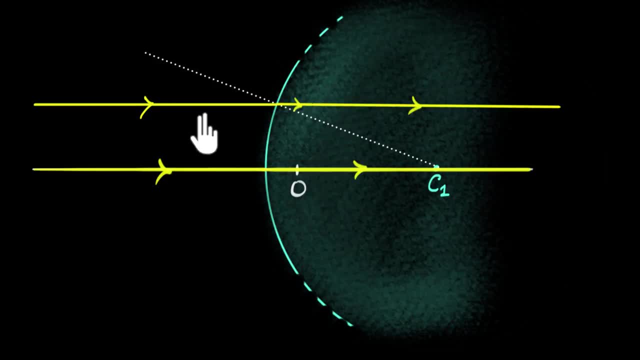 low is a denser medium, and so the ray of light is moving from rarer to denser. the ray of light is going to bend towards the normal. so this ray will bend somewhat like this, towards the normal, and these two rays are going to meet somewhere over here. let's call that point as i. that's where the 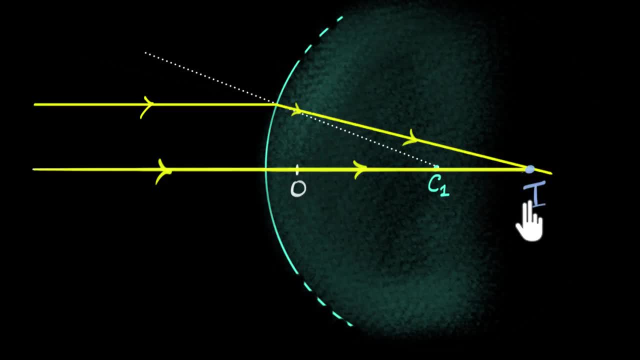 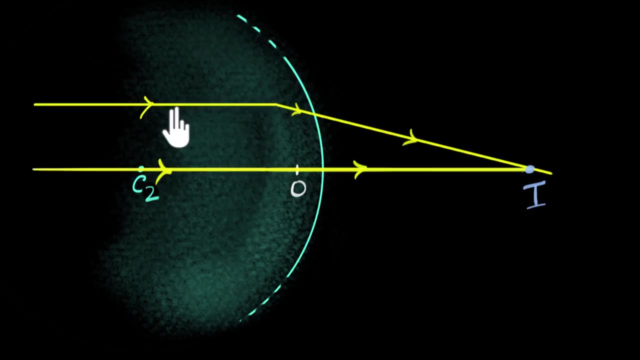 image is formed, but of course this is not the final picture, because we haven't considered the second surface yet. so this is the image if the second surface was not there. so now let's consider the second surface. now for the second surface. this is the incident ray we can totally neglect. 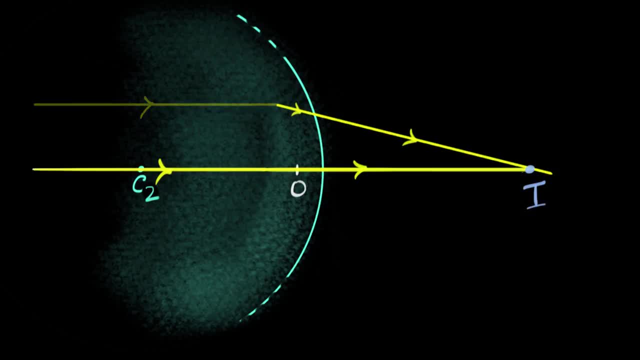 this initial incident ray. and so again, if you draw a normal, then notice this ray of light is now going from the denser medium to a rarer medium and so it's going to bend away from the normal. so here's our normal. so this ray, after refraction, is going to go away, bend away from the 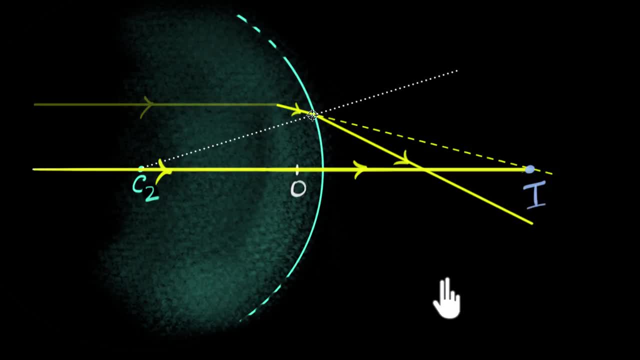 normal and as a result somewhere over here maybe, and as a result notice that the initial two parallel lines. they are not meeting, so the istir two parallel lines are affecting the coax cam. anybody saying to be happy, please stop doing that and create a feature in the comment section for less ЗИ. 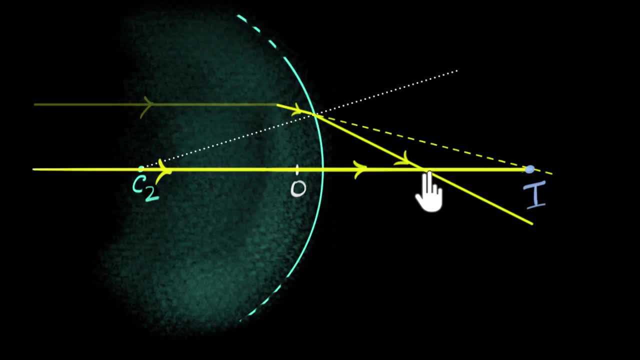 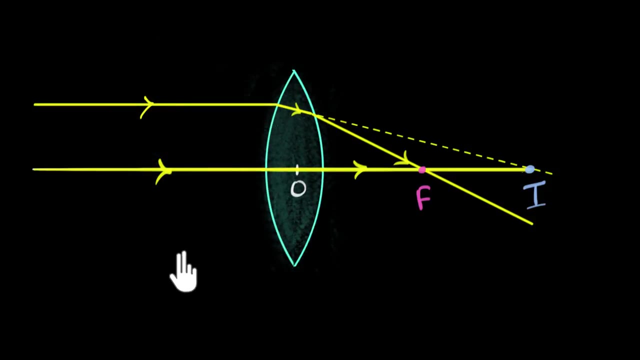 rays are being focused after refraction, finally, at this point. so this is our principal focus. so here's our principal focus, and this distance from here to here is the focal length. that's what we have to figure out. so how do we figure this out? well, since we are dealing with refractions at curved surfaces, we'll 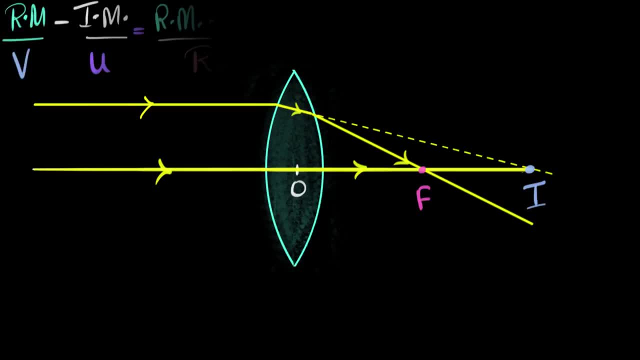 have to use, no surprise, the curved surface formula. so this is how I like to remember the formula. RM is the refractive index of the refracted medium, meaning it's a medium that contains the refracted ray. similarly, IM is the refractive index of the incident medium. again, it means the medium that 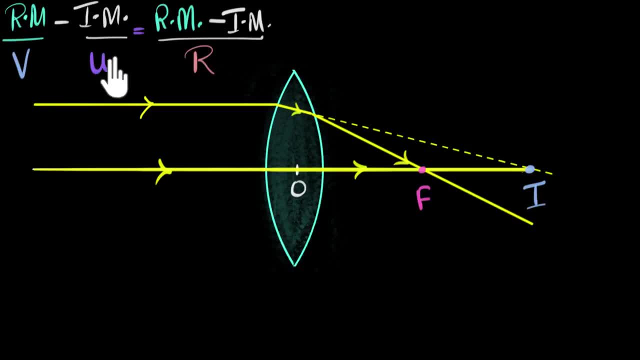 contains the incident ray and V is the image distance, U is the object distance and R is the radius of curvature. and since we have two surfaces, we'll have to apply this formula to each of this surface. so let's start with the first surface when we apply this formula to the 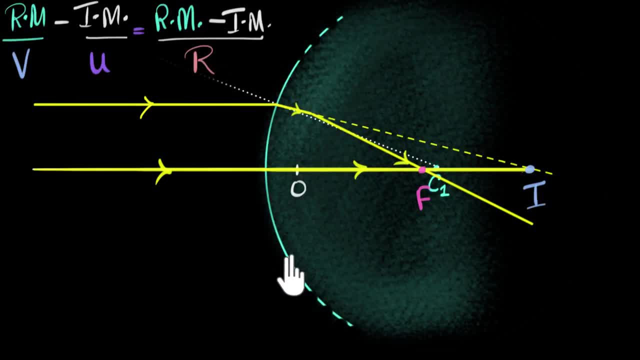 first surface, we are going to absolutely neglect the second surface. that means we are going to neglect this refraction that's happening to the second surface and we'll assume that the two rays are actually going to meet up at this point. and that's the trick to solving problems. when we have multiple surfaces, we only 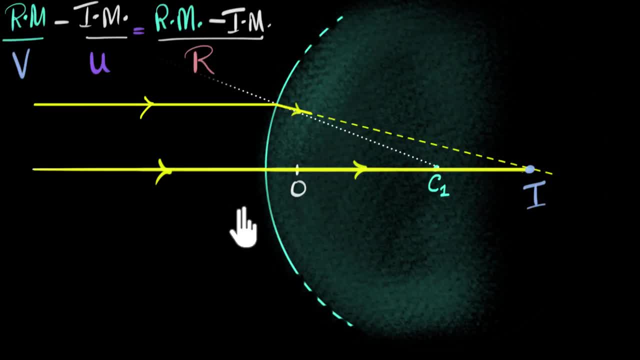 consider the first surface, ignore all the other surfaces. alright, now let's apply this formula. alright, the refracted medium is the medium that contains the refracted ray that's over here. so it will be this medium. let's say, its refractive index is N2 and the incident medium will be the. 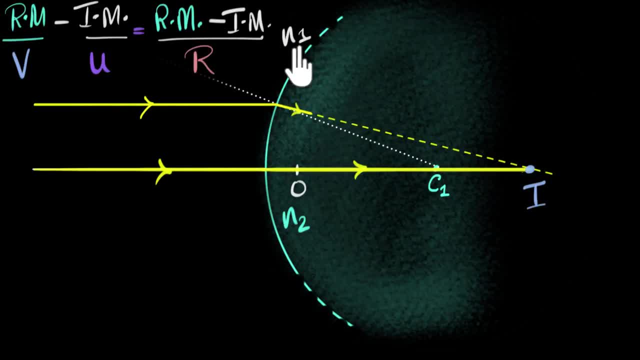 outside medium, because this is the incident ray and let's say, its refractive index is N1, so let's substitute that over here. so the refracted medium, that is N2 divided by V, which is the image distance for the first surface. this is the image, so the image distance is going to be this distance. now, 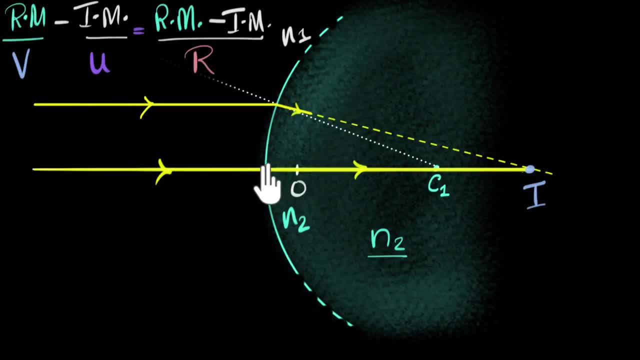 since our lens is thin. whether you consider the distance from this point or consider from this distance, isартic distance isin the other side. so if you this point, it's not going to matter. So it's the same thing. That's the whole reason. we're dealing with thin lenses. 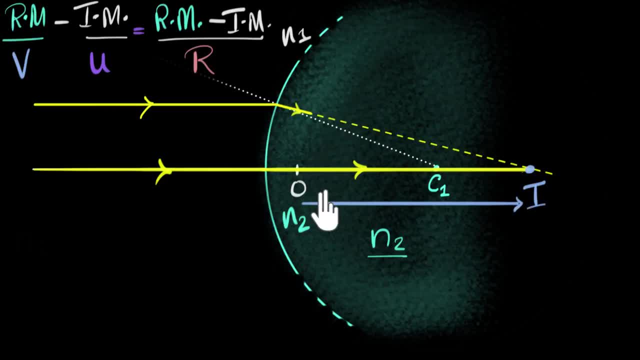 So this is the image distance V. It doesn't matter where you take it from, all right, So this is the image distance V. So it's going to be N2 divided by V minus the incident medium, That's, over here, the outside medium. 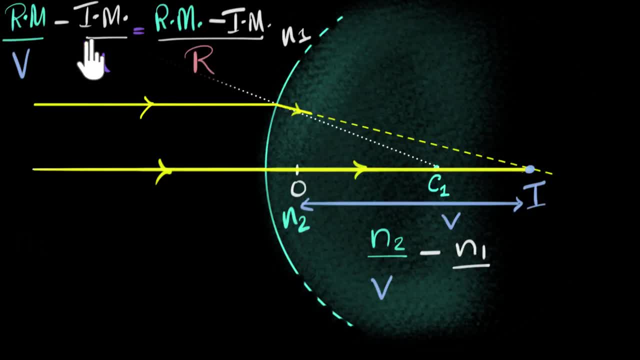 That's N1.. N1 divided by U, the object distance. Well, where is the object? Well, there is a flight of paddle, And so the object is far away. That means infinity. So we could say: object distance is infinity. 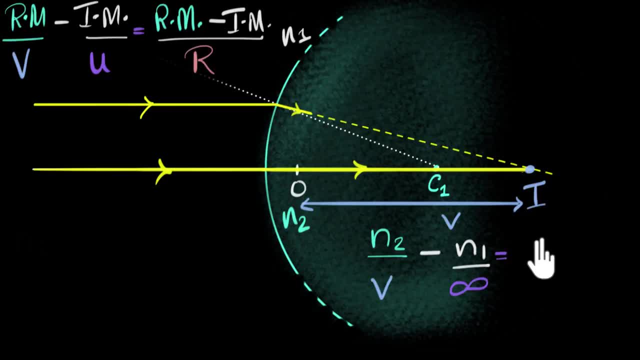 That's going to be equal to this minus that. So that's going to be N2 minus N1, minus N1 divided by R. Well, what's R? R is the radius of curvature of this surface, And since this is the first surface, 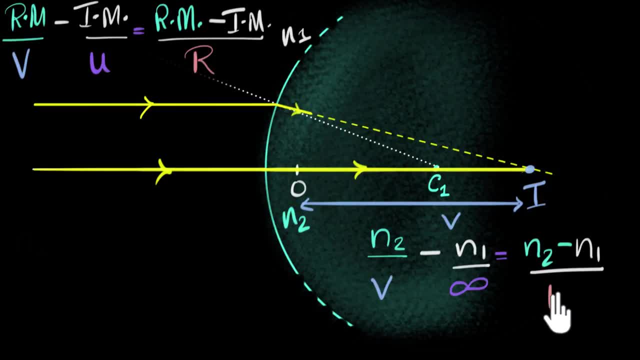 let's call that radius of curvature as R1, R1.. You may be curious As to why we're not using sign conventions at all. We'll talk a little bit more about that later on, But this is what we got for surface number one. 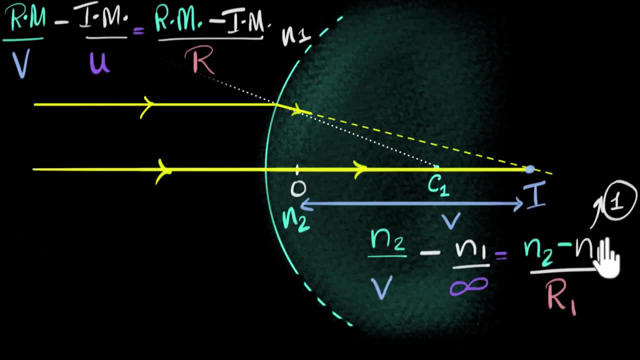 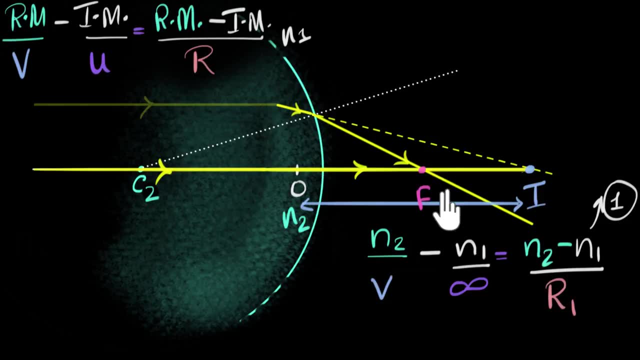 Let's call that as equation number one. Now let's apply the equation to the second refracting surface, And so for the second surface, after a fraction, the image is formed over here, And so now we have to apply this formula for the second surface. 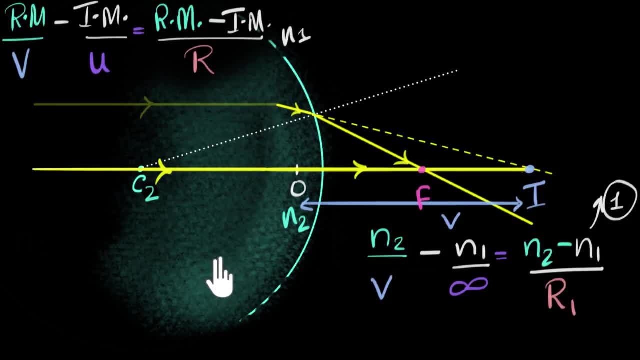 It'll be a great idea to pause the video and see if you can try this yourself. All right, let's do this. Okay, again. refracted medium. This time- notice- refraction is happening in the outside medium, So this time the refracted medium is N1.. 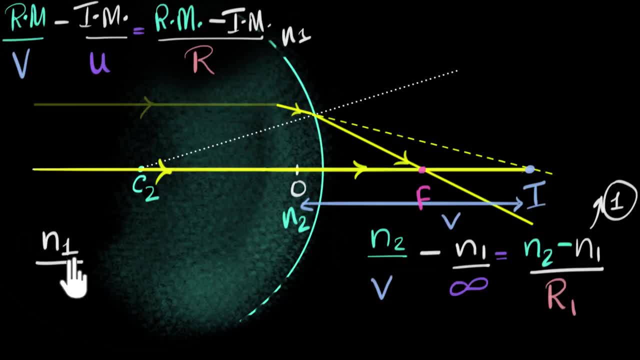 So we'll get N1 divided by the image distance. Well, our image now is over here. Think about this: For this surface, this is the image And the image distance itself is the focal length. So, divided by the focal length, F minus the incident medium. 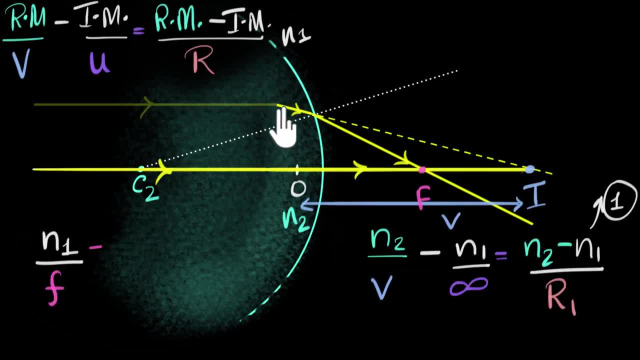 The incident medium. Well, this is the incident, And therefore now the incident medium is the medium of the lens, And so the incident medium is N2 divided by the object distance, And we might think: well, the object distance is infinity right. 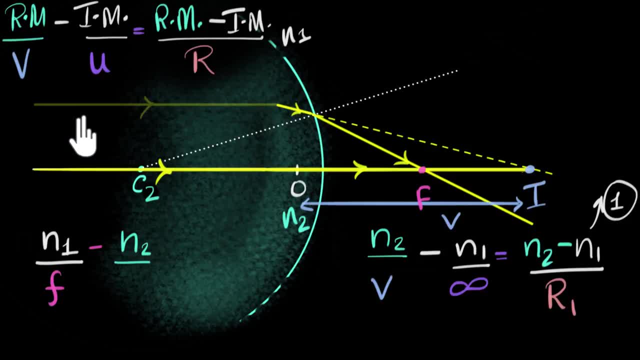 Well, no, we have to be very careful, And this is the important part, You see, if when you consider these incident rays, that's when the object is at infinity. But these are the incident rays for the first surface. For our second surface, we got the radius. 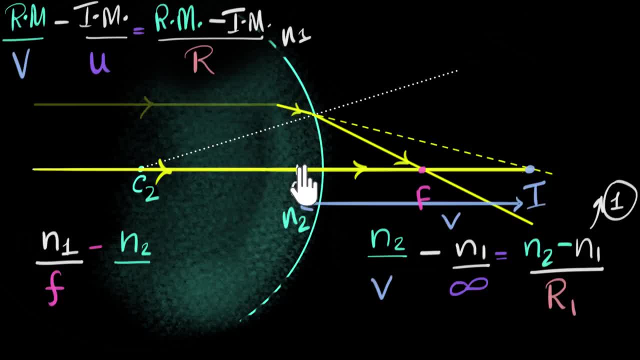 these are the incident rays And here's how I like to think about it. Object is where the incident rays meet. Simple, all right. So, for example, if here was the object, then if we drew incident rays like this, incident rays like this: 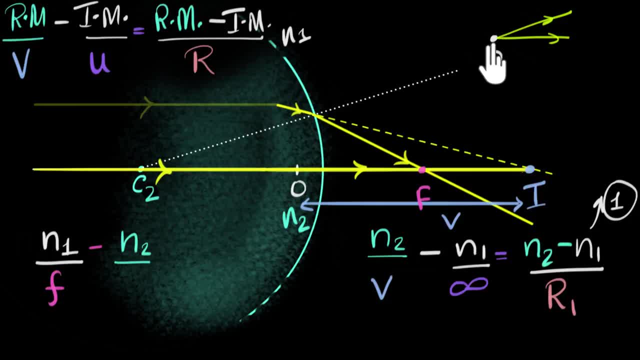 wherever the incident rays meet. that would be our object, isn't it? So we just have to ask ourselves: where are these two incident rays meeting? Well, if you backtrack them, they're not gonna meet anywhere, But if you go front, they are meeting at this point. 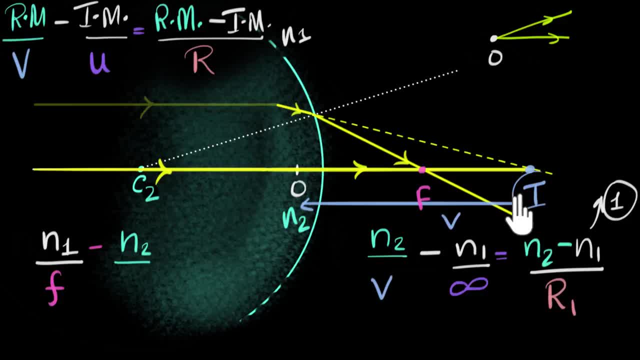 And it's for that reason this is going to be our object. Now, I know it sounds a little weird to call that as an object, because the rays of light are not really meeting at that point. They would have met if it wasn't for this surface. 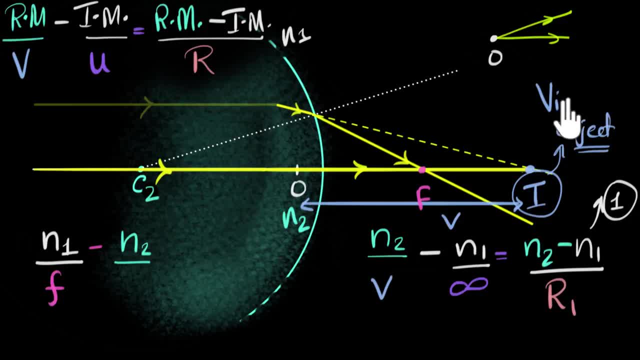 So we give a name to such kind of an object. We call that as a virtual object, as a virtual object, But you don't have to worry too much about that. Nevertheless, it's the object for our second surface, And this is the general way. 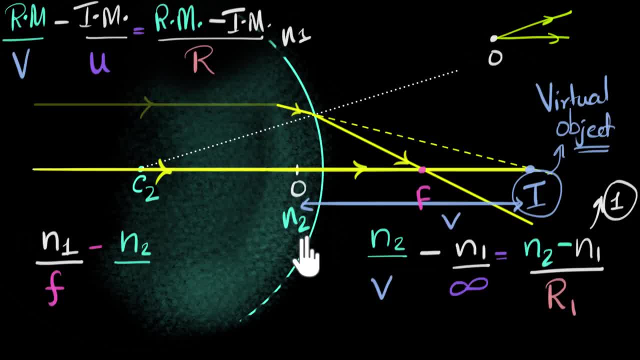 in which, how we we solve any problem with multiple surfaces, The image for the first surface acts like the object for the next surface. This is the general way to do problem solving. So, anyways, this is our object for second surface, And so our object distance will be v. 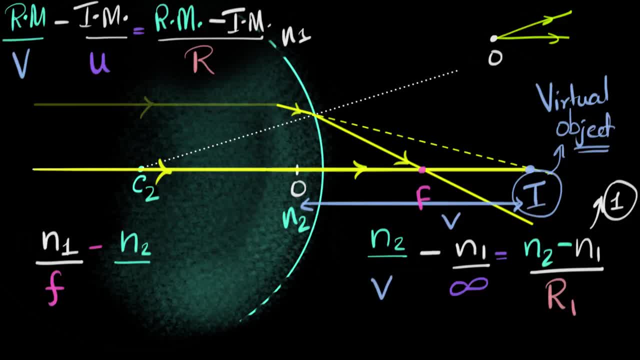 Whatever was the image distance before now, that same is our object distance. all right, So this is going to be our object distance, And so that will be equal to. we have to do n one minus n two, So n one minus. 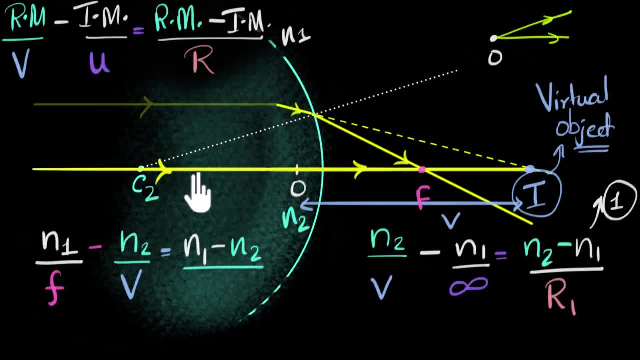 minus n two, divided by the radius of curvature, the radius of curvature of this surface, that need not be the same in general for the radius of curvature of the other surface, And so we can write as divide by r two, And this now is our equation: two. 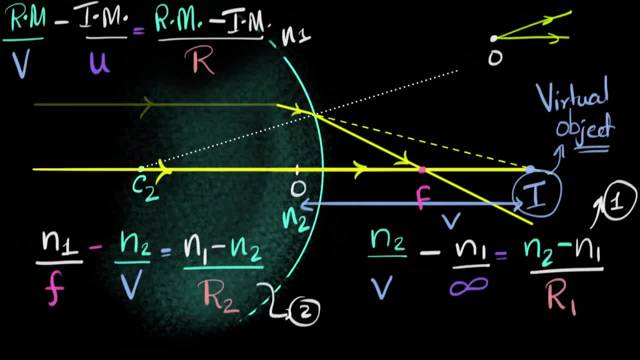 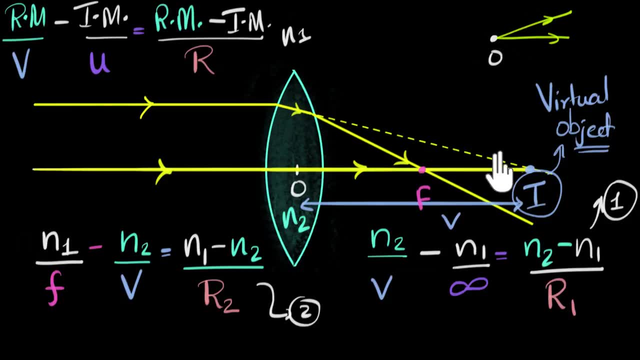 equation for the second surface. And so now, if you look at the final picture, in reality these rays of light are actually meeting up at this point. This was something that we just cooked up, assuming what would have happened if this was not there. 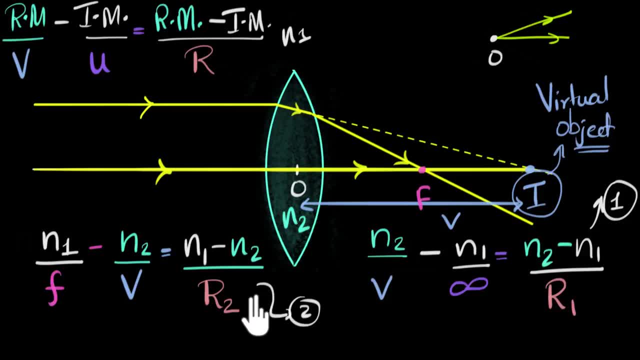 So this v is something that we cooked up and we shouldn't have that in our final equation, And so somehow, by using these two equations, we can get rid of v. In fact, if you look carefully, you have a negative n, two by v here. 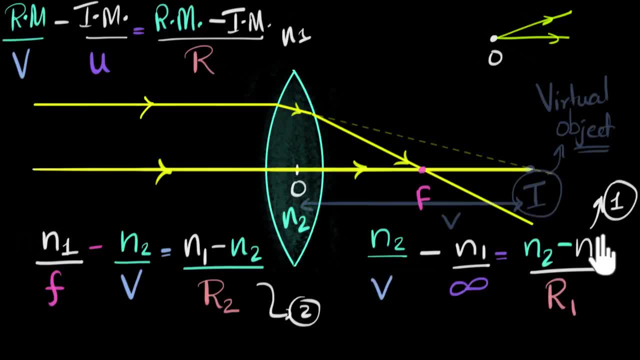 you have a positive n, two by v here. So if we just add the two equations, the v cancels out, and then we can figure out what the focal length is. And so, again, it would be a great idea to pause the video. 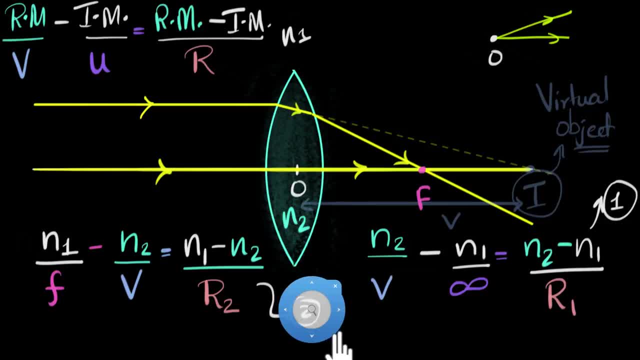 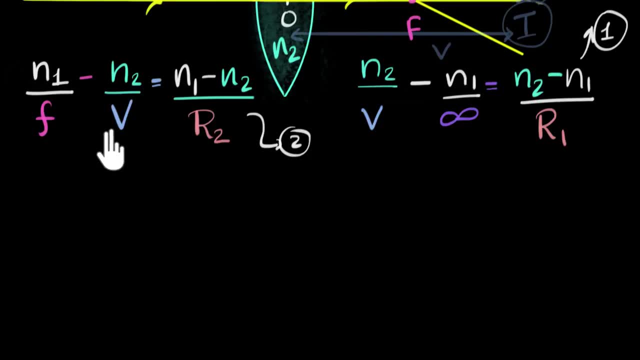 add the two equations and see what you get. All right, let's do that, Let's make some space. All that is left is now algebra. So if we add the two equations, these cancel out. So on the left-hand side, 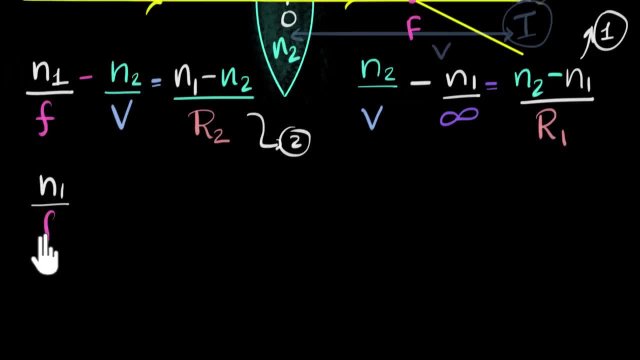 we are left with n one divided by f, minus n one over infinity. What's n one over infinity? One over infinity is zero, So n one over infinity is also zero. So this gap goes. So all is left is n one over f. 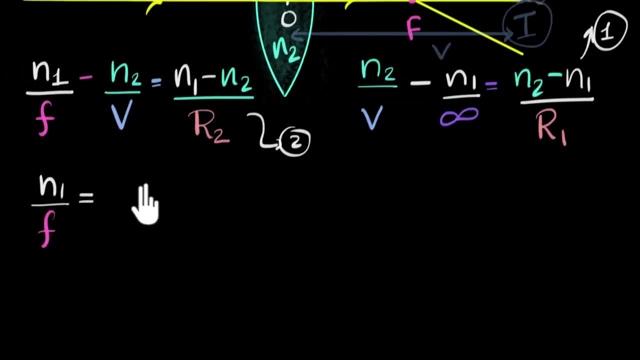 that's equal to- we're adding these two right, So that'll be n one minus n two divided by r two plus n two minus n one, n two minus n one divided by r one, And so finally we can simplify that. 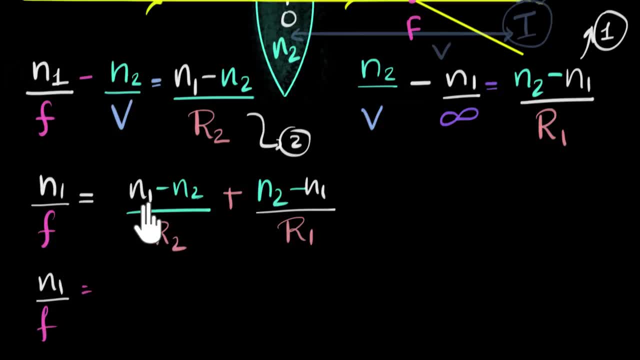 Not. finally, there might be one more step in the world. over there We can take n two minus n one common, So let's do that. So if you take n two minus n one common out from here, we end up with one over r, one over here. 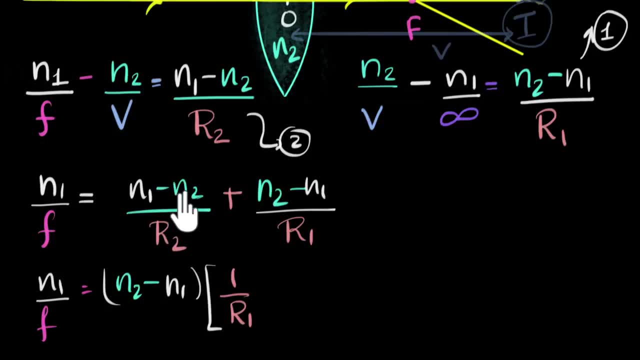 one over r one. And notice, since we took n two minus n one common, there's a negative one that remains over here. So you get negative one one over r two. Just think about this for a while. I just picked out n two minus n one. 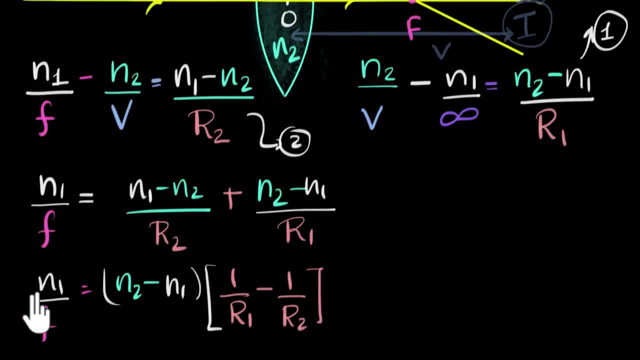 so a negative one remains, And so, finally, we can divide the whole equation by n one, And so this goes from here and n one comes over here And this. now we can treat this as our final equation, grand equation that gives us what the focal length is. 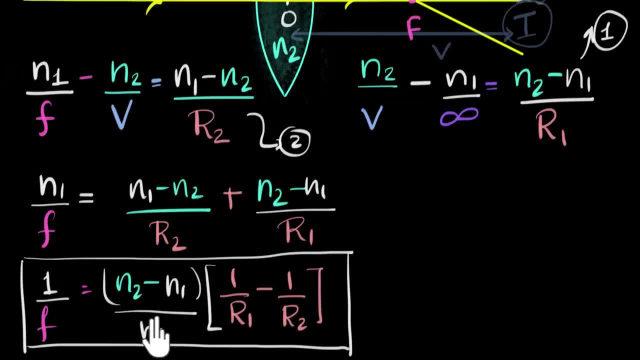 And if you look at this carefully, in fact, you know what we can make. one more simplification: We can divide each term by n one, and so I'll just do that over here to save space. You'll get n two by n one. 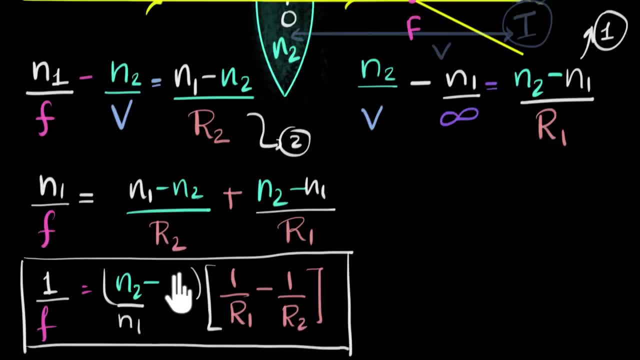 minus n, one by n, one, that is just one. all right, So excuse this, because I was running out of space. So this is the final equation that tells us what the focal length is and you can see that depends on the refractive indices. 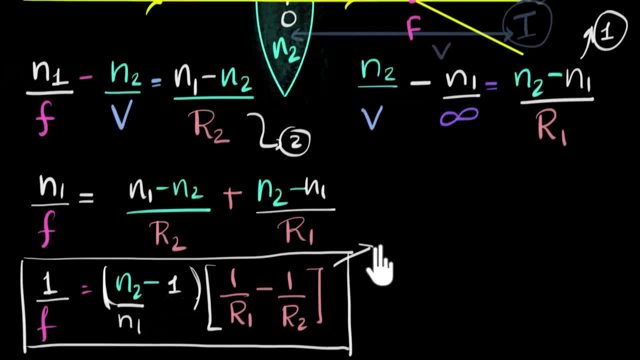 and the radii of curvature. And we give a name to this equation. We call this as the lens makers equation or lens makers formula. It's called lens makers because tomorrow, if you want to make a lens of a suitable focal length, 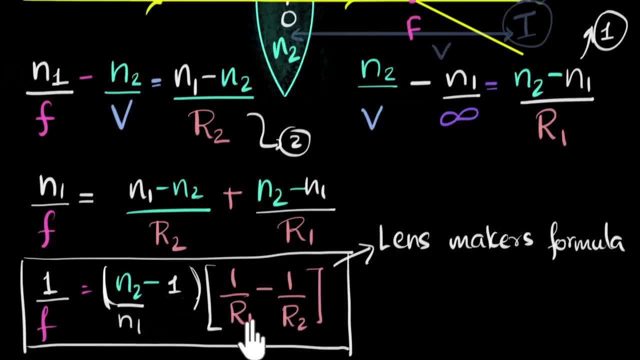 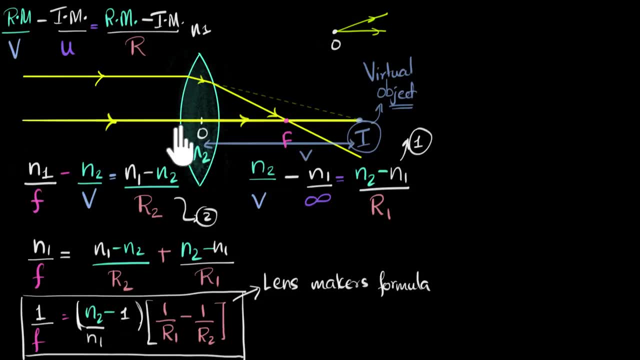 then you can use this equation and choose appropriate values of n two, n one, r one and r two. So, to quickly summarize, here are the key takeaways of this derivation, Since we're dealing with curved surfaces, for each surface. 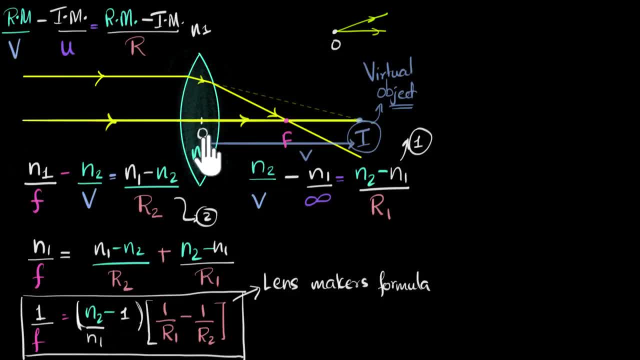 we're going to use the curved surface refraction formula, Then the image of that first surface is going to be the object for the second surface. Then you put together the equation and we end up with this final result. One last question we might have is: 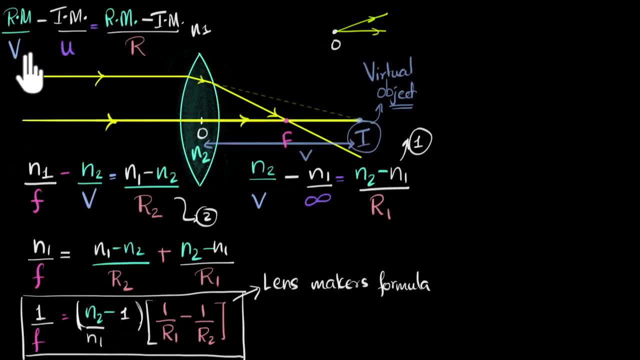 why we haven't used sign conventions when we substituted in this curved surface formula. Well, think of it this way: This is a general formula which works for any case when it comes to curved surface refraction. Now, if we were solving in numerical, 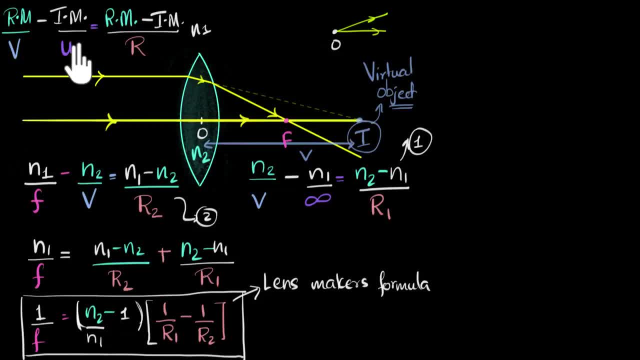 which deals with specific cases, then we would have substituted using signs. And that's what we always do When we are solving numericals: we always substitute signs. which means, whenever you substitute numbers with signs in a general formula, you end up solving for that specific case.